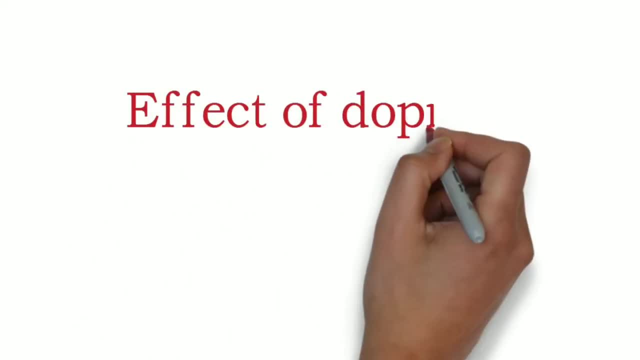 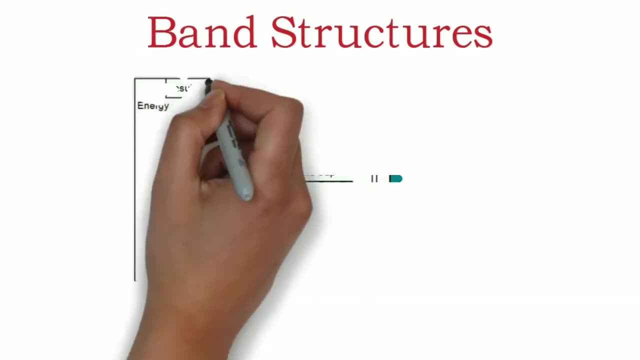 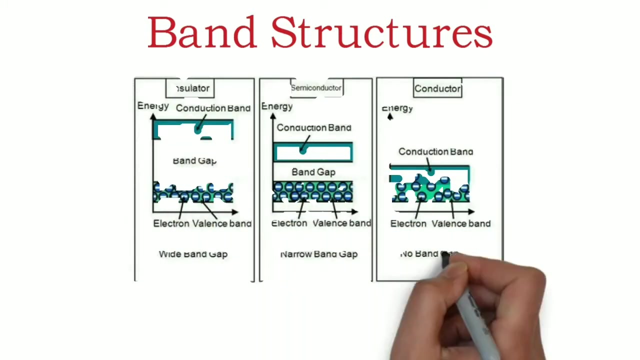 In this video I am going to discuss about the role of doping in band structures. Before knowing the doping in band structure, we must know what are the band structures. Band structures are classified into three different types. They are insulator, semiconductor and conductors based on the energy gap between balance band and conduction band. 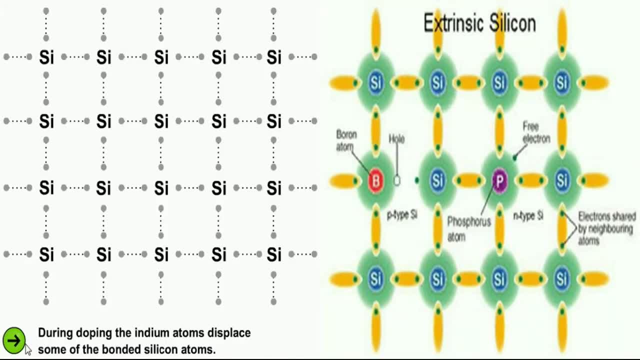 Here in these semiconductors. these semiconductors are classified into two types again. They are intrinsic semiconductors and extrinsic semiconductors. In this doping of band structure, we will be speaking about only the extrinsic and intrinsic semiconductors. 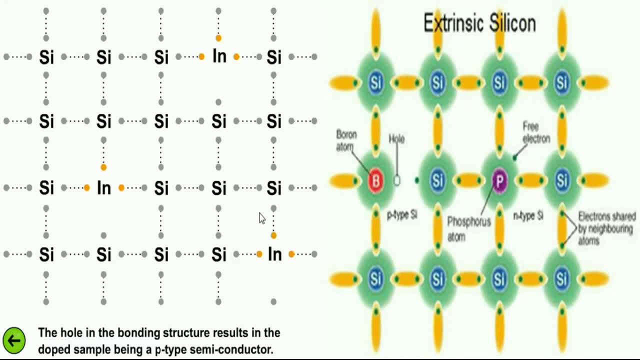 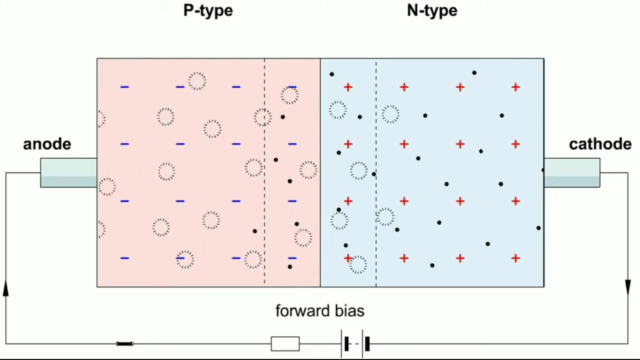 Here these extrinsic semiconductors are again classified into two different types. They are p-type semiconductors and n-type semiconductors. Now let us discuss what is intrinsic semiconductors If the Fermi energy gap is small between the balance band and conduction band. 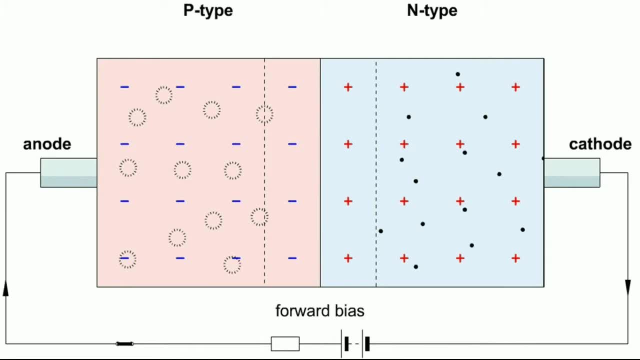 the electron from balance band is exited to conduction band. It is called intrinsic semiconductors. Both the holes left in balance band and exited electron to conduction band contribute to conductors. As the temperature rises, the number of electrons promoted to the conduction band increases. 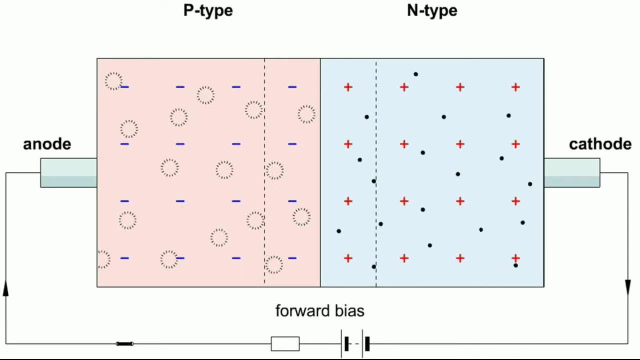 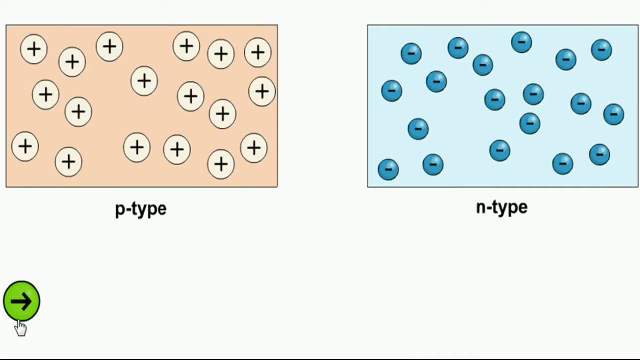 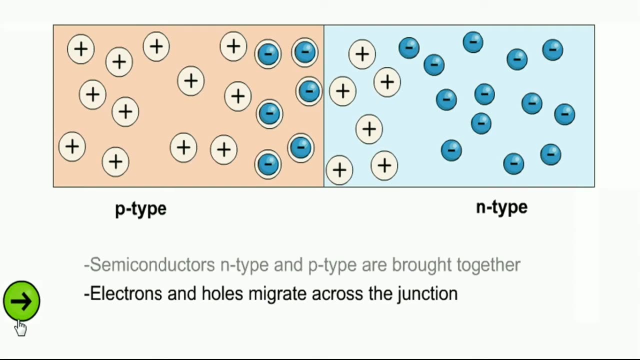 contributing to increase in conductivity of semiconductors. Now let us discuss about extrinsic semiconductors. If the Fermi energy gap is more where the electron cannot be exited to conduction, band conduction can be improved by introducing an impurity into the semiconductor material. 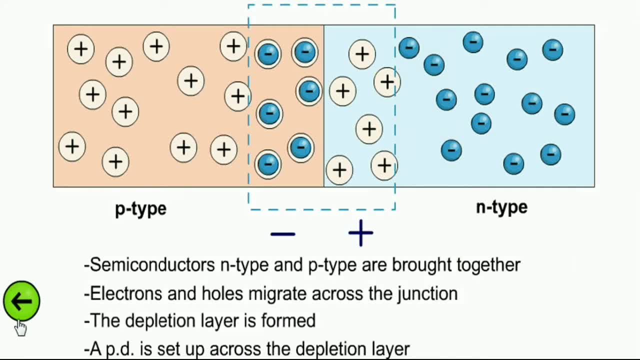 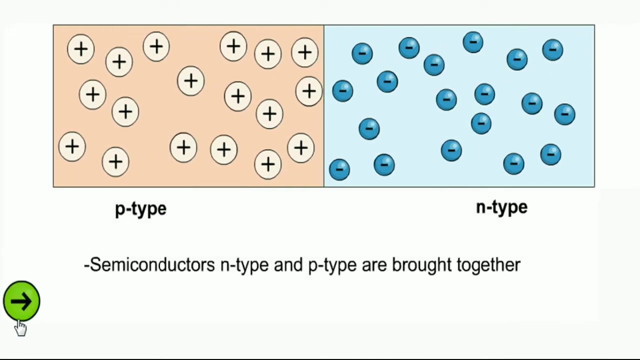 which is called a doping. Doping can be carried out by introducing an electron deficient or electron rich impurity into the material which produces p-type and n-type semiconductors respectively. The impurity form an impurity bond, called donor bond, between balance band and conduction band of the material. 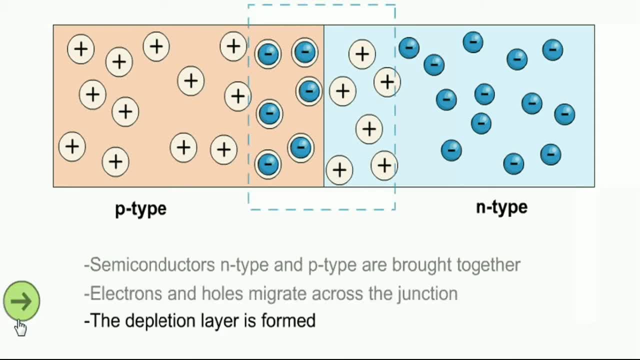 whereby Fermi energy gap is reduced And conduction takes place Like this extrinsic. semiconductors are classified into two types, as I have already told earlier. They are n-type semiconductors and p-type semiconductors. 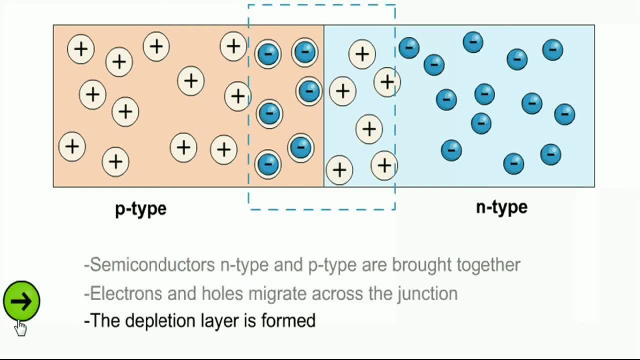 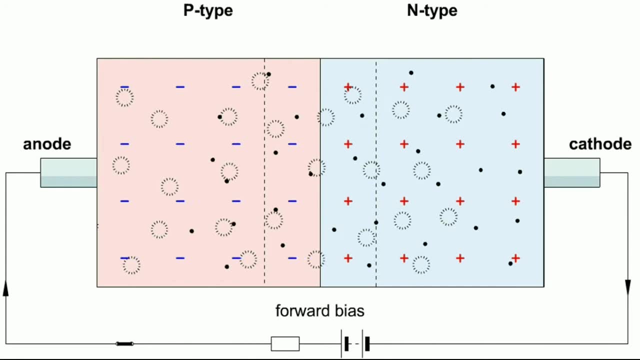 Now let us discuss about n-type semiconductors. N-type semiconductors are produced by doping. silicon or rhenium with pentavalent impurity atoms like phosphorus and arsenium, etc. A minute amount of rhenium is produced by doping, silicon or rhenium with pentavalent impurity atoms like phosphorus and arsenium, etc. 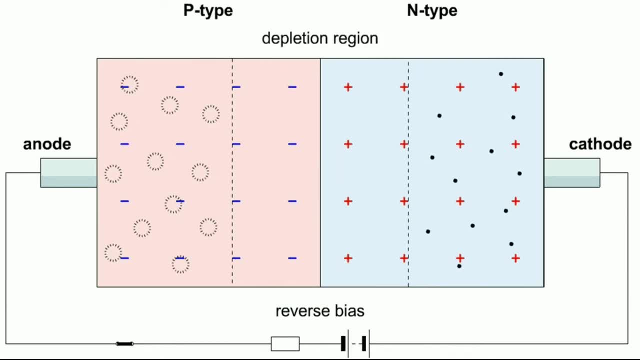 A minute amount of silicon or rhenium atoms are replaced by phosphorus, with five electrons in its outer shell. From this, what we can able to understand, It will be having five pentavalent electrons. There must be five vacant electron atoms should be attacked in these bands. 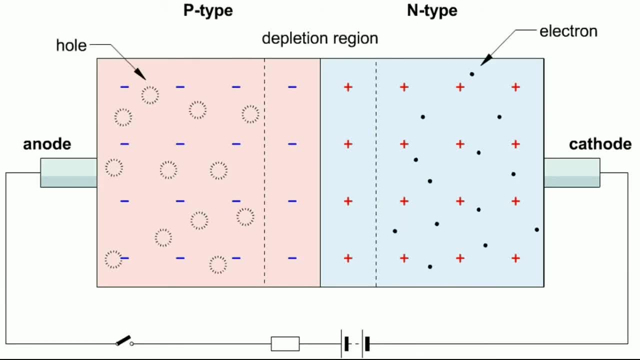 Only four electrons form covalent bond with silicon or GE, And fifth electron is localized at absolute zero At the normal temperature. some of the fifth electron of impurity are promoted to conduction band, causing conduction, Since the conductivity of such conductors are due to negative electrons. 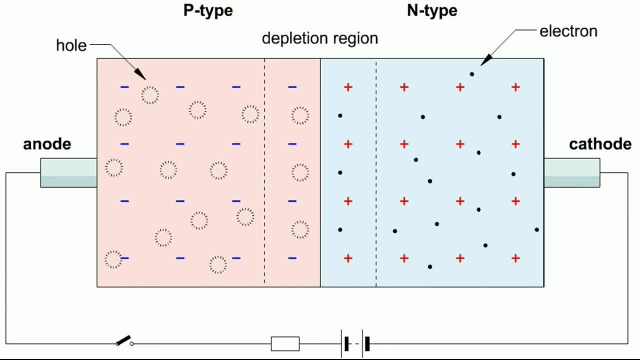 they are called n-type semiconductors. Now let me discuss about p-type semiconductors. By introducing a trivalent impurity atom, like aluminum, boron, gallium, into silicon or germanium, the replacement of these silicon or germanium atoms by impurity produces an incomplete bond in the structure, producing a positive hole. 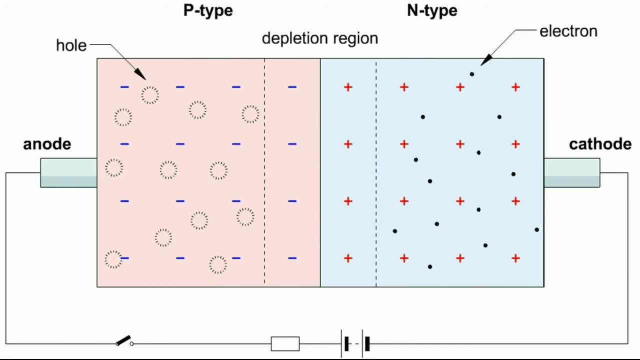 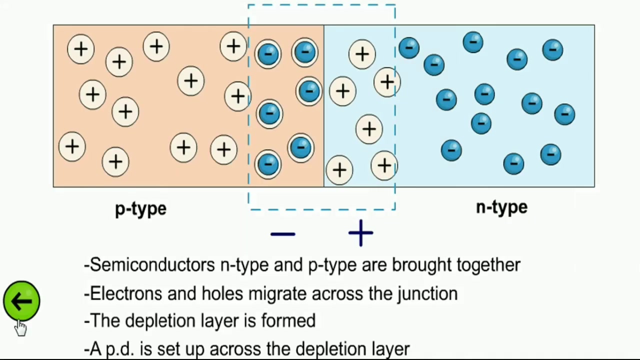 The positive holes are replaced around the trivalent impurity atom at low temperature or absolute zero At normal temperatures. the valence electrons on the adjacent silicon or ellenium atoms may gain sufficient energy to produce into the hole, thus creating a new hole on the silicon. Thank you for watching.